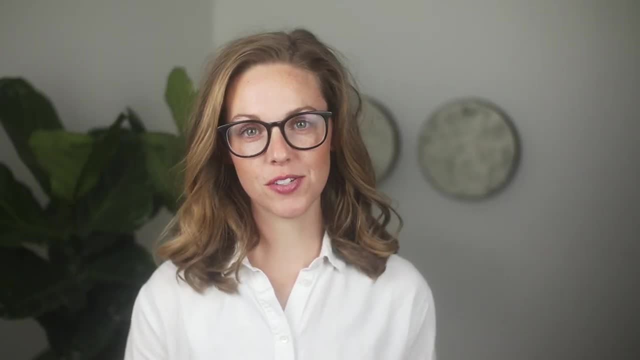 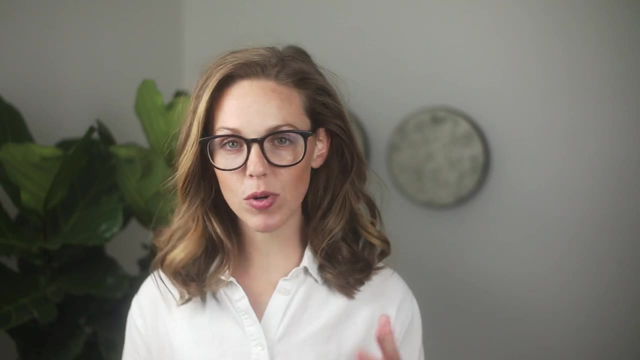 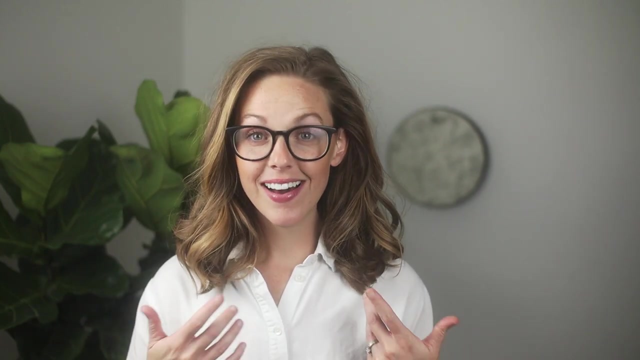 Hi there, my name is Victoria Bowler, and today we are talking about some options for structuring the music lesson. In a typical music class, we might see students between 25 and 45-ish minutes, So within that time frame, what is the most impactful way to organize our time? Ideally, we would be: 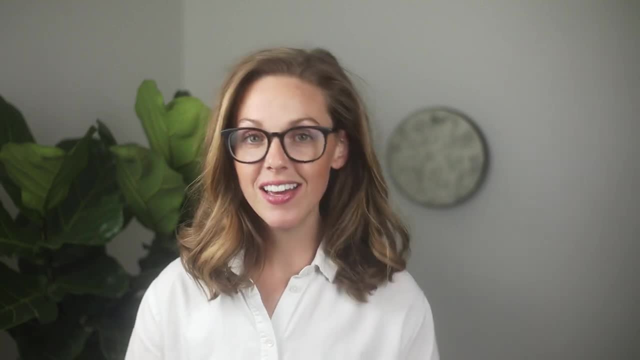 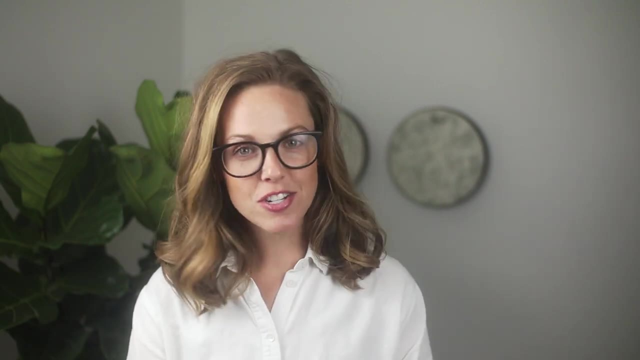 dividing class up so that students have the highest amount of fun and engagement and then the highest amount of musicking as possible. That's what we'll talk about today. Conversations around how to organize daily lessons are curricular conversations, And in the podcast that goes. 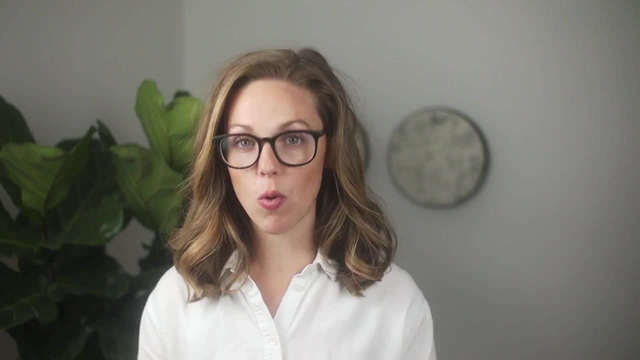 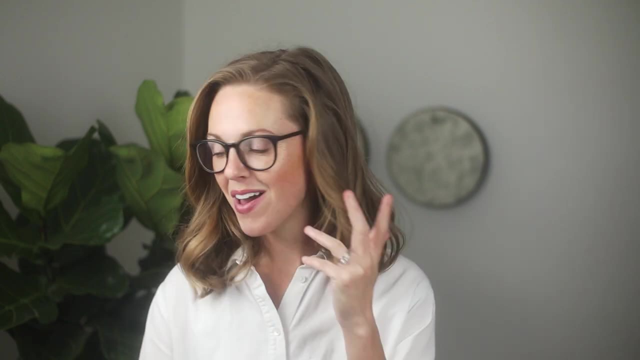 along with this video, we talk about some different frameworks for organizing curriculum. So if that is something that is interesting to you, you can use the link in the description to take a listen. All right, with that said, let's jump in. Let's start with the first lens. What? 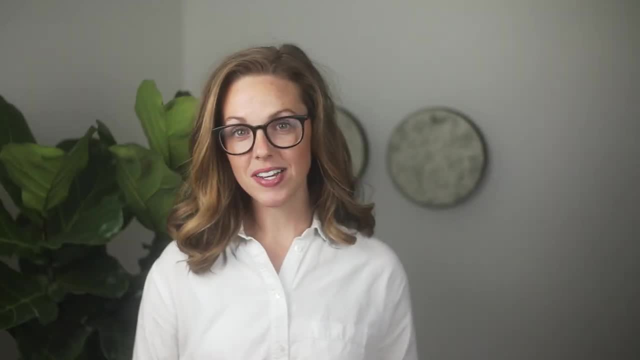 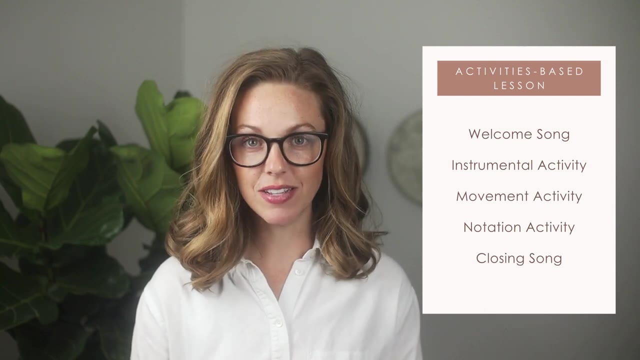 are we going to do? One very popular option is to organize the lesson plan around activities. For this, the breakdown of the lesson might look like a welcome song and then an instrumental activity and then a movement activity and maybe a notational literacy activity and then a closing. 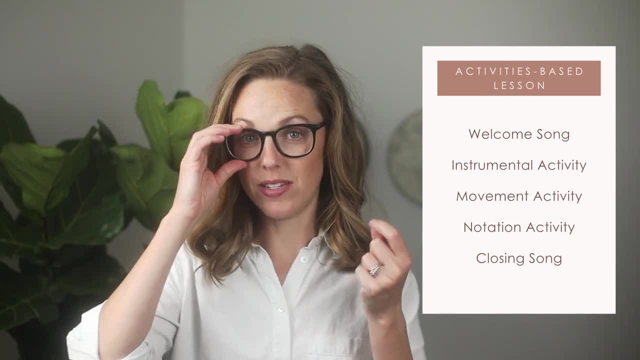 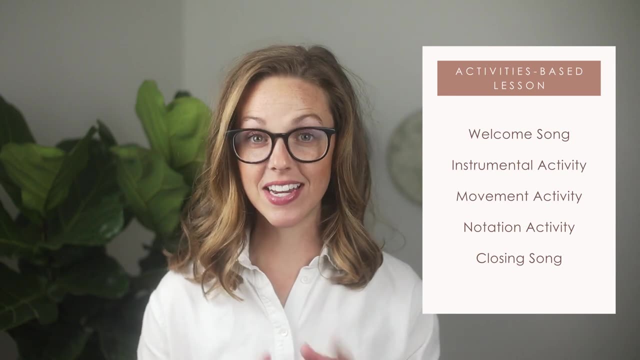 song. This lesson plan is based around the doings of music, or the musical skills. There are some really positive things about this lesson structure that I think are worth highlighting, namely the different modes of musicking that are happening here. This lesson is set up to be: 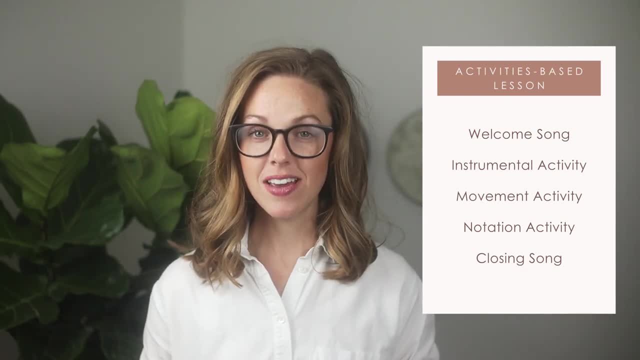 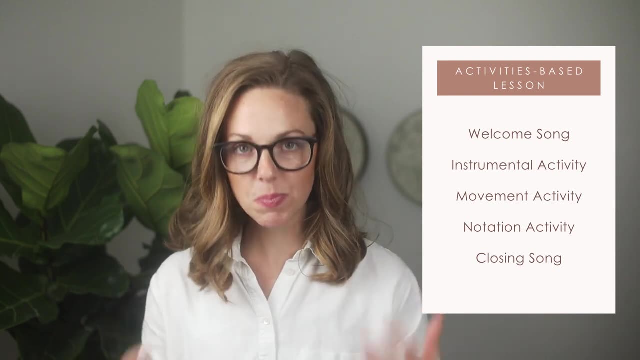 incredibly active and to keep students engaged the whole lesson. So notice that we're not staying on one skill throughout the whole lesson, We're jumping around. we're moving around to different ways to experience and understand music And you might recall that, within the lens of multiple means of engagement, this is a really 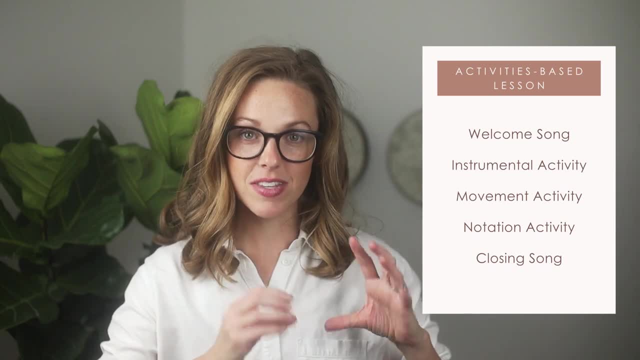 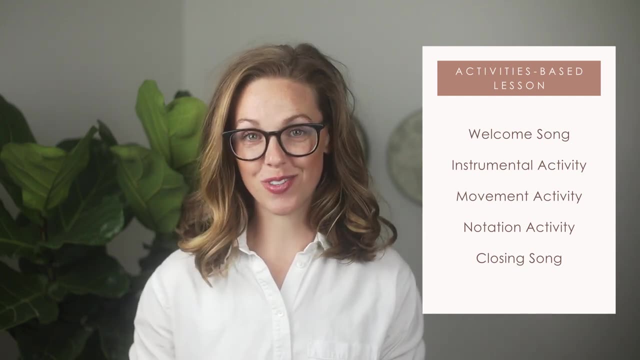 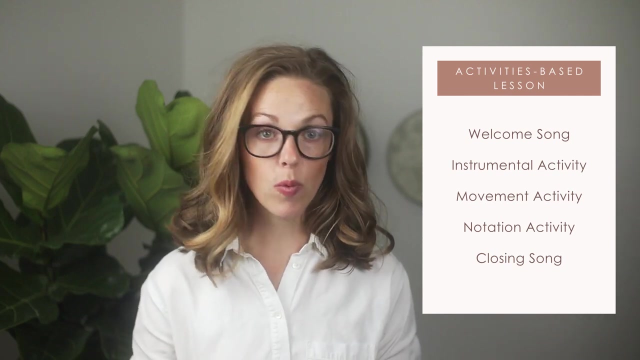 beautiful way to structure the lesson. The diversity of the experiences is really the gem of this lesson structure. in my opinion, There are some potential challenges with this approach, though, If we exclusively organize lessons around activities like a welcome song and an instrumental activity, that kind of thing. 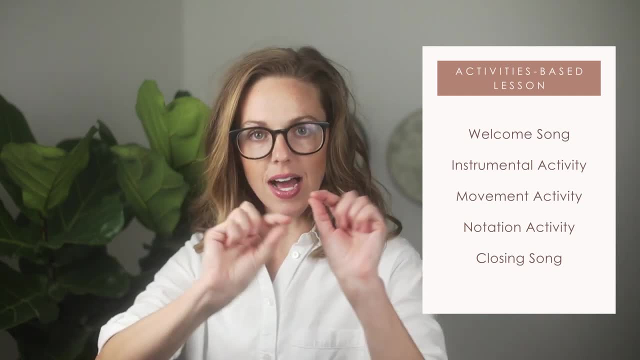 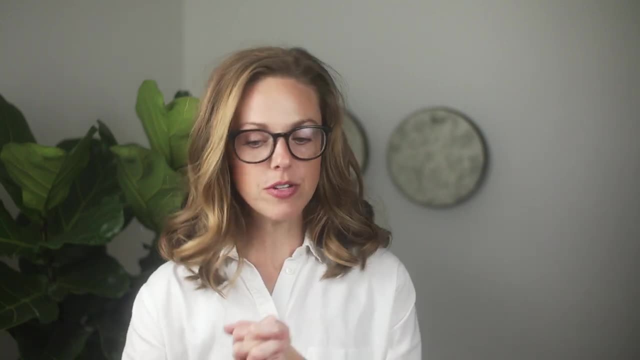 it can become tricky to see the thread that ties those activities together from week to week. So here's the problem. Let's imagine that you are searching Pinterest for a fun activity for third grade and you find one, and you use it in class and your students love it Well. 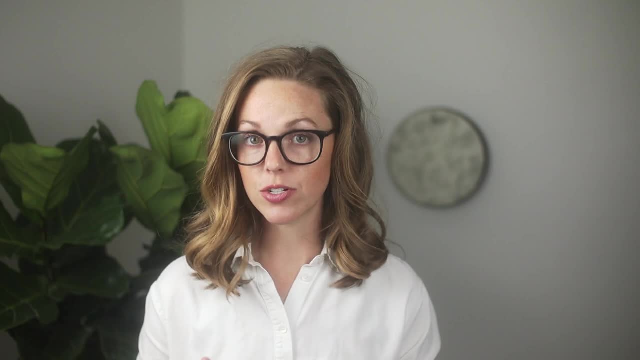 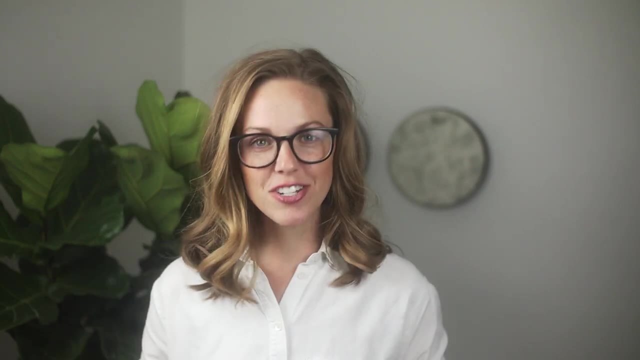 that's great, That's a win right. But the problem here, potentially, is that when the fun activity is over, what are you going to do in the next lesson If I teach you how to play a song on barred instruments and that's it? 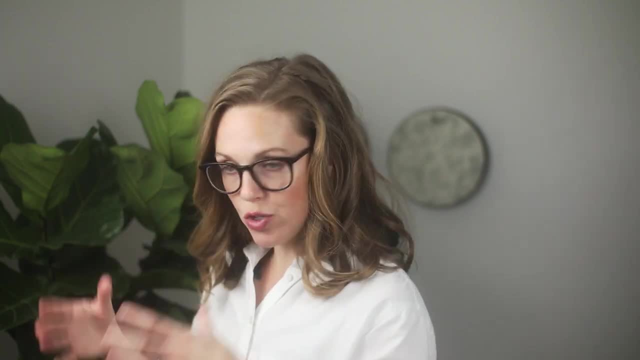 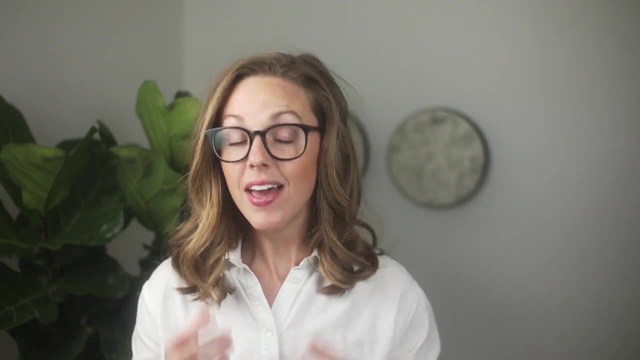 that's the entire lesson segment, then the next class. I need to find a new song to teach you. You see, we're constantly starting over on this hamster wheel. We're starting over from scratch each lesson. And then what happens if I am teaching a mallet part but someone doesn't? 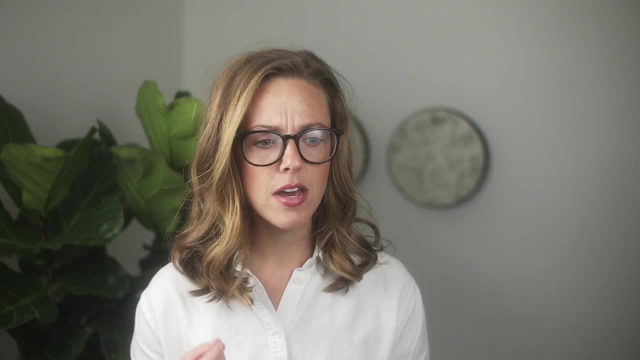 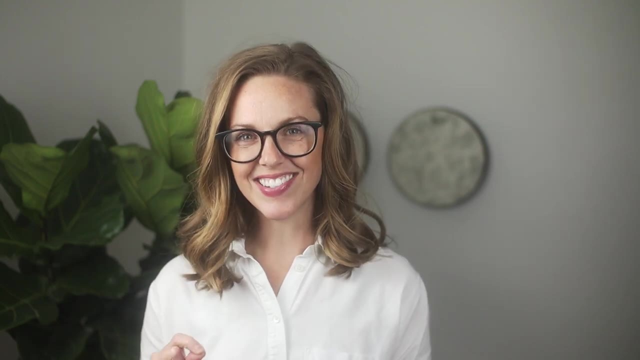 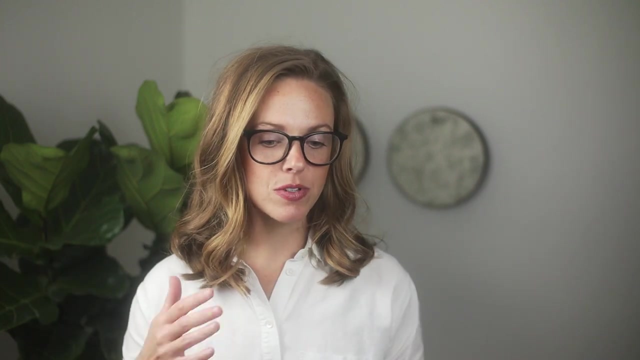 understand what they are supposed to be doing. They don't understand the specific part that they are playing. What are we doing to help students build knowledge and skills that they can reference when they come against a new challenge? Where are the instrumental skills that we could? 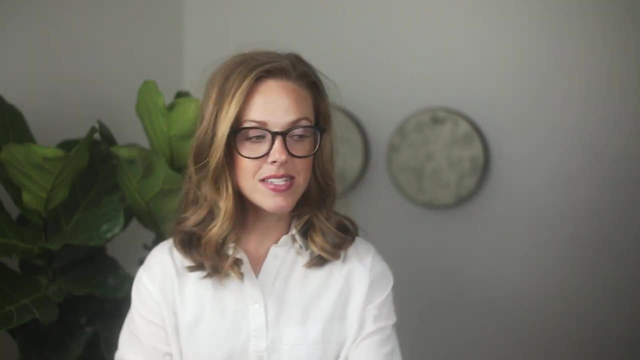 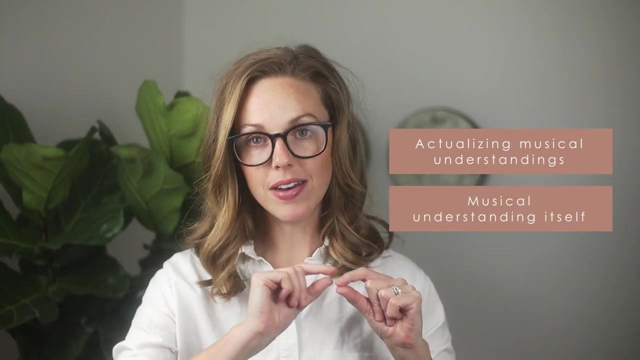 build off of in this example. So this is a lesson structure based on how we experience musical understandings. What we're not explicitly addressing here is the common thread of the understanding itself from lesson to lesson. So let's think about a way we might take this. 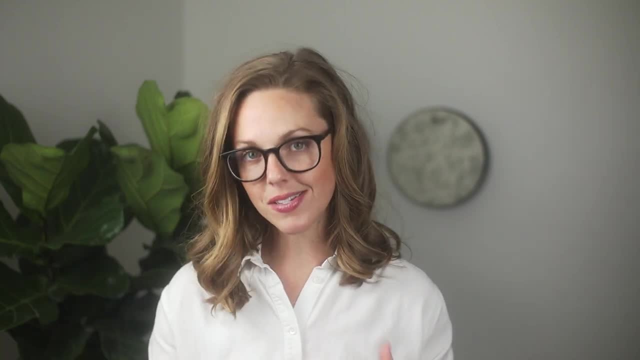 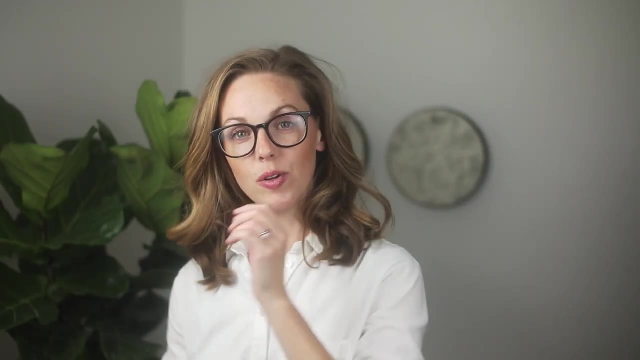 active approach for this lesson structure and tweak it with a slightly different framework. So here's another example, And this time it's based around what we will learn instead of what we will do. We're going to start off with a welcome song and then move to a main musical focus, and then we'll have a game or a change of. 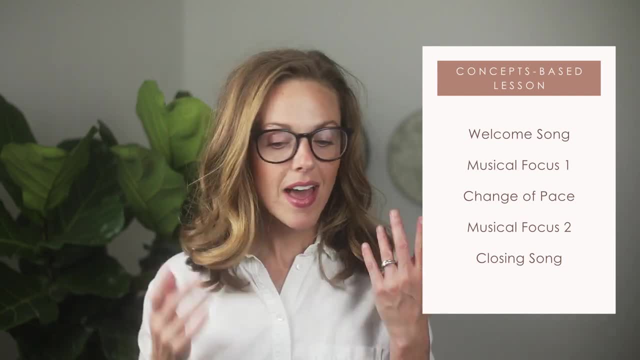 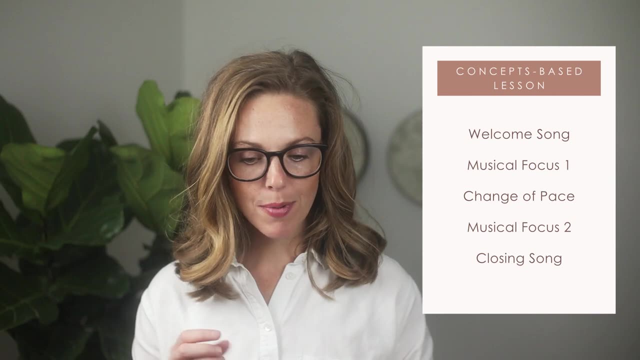 pace and then a secondary musical focus and then a closing song. And I should reference here that this framework is not something that I invented. This is an established way to organize the lesson, and I read about it first in Susan Brumfield's work, but you can find it in other places in 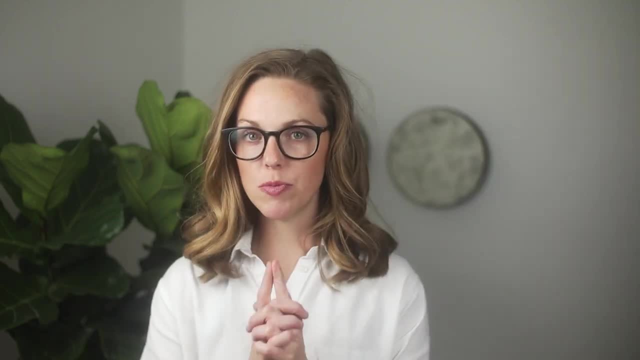 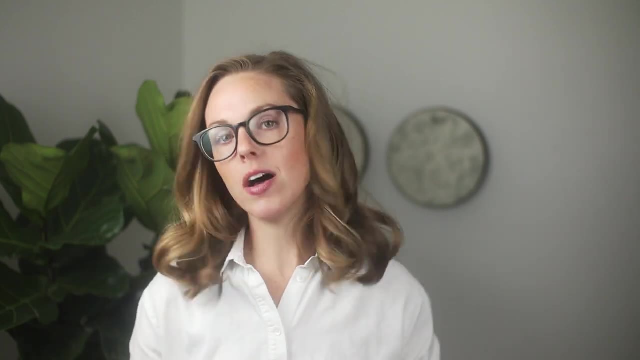 music pedagogy conversations. Okay, so let's just take that first musical focus. Let's imagine that the musical concept we're working on- because, remember, this is a concept-based approach- let's imagine the concept is pitch and then the specific tonal pattern is law and so law. so me. 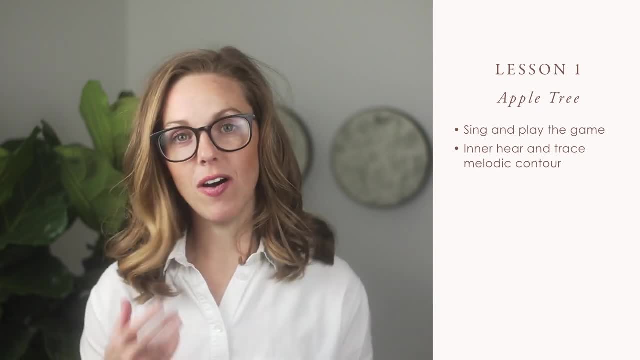 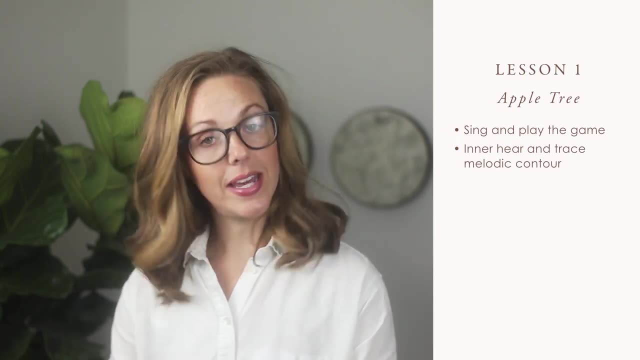 In the first class we might spend like seven minutes with the song Appletree in that main concentration section. So let's say that students are going to sing the song and play the game. It is likely that we will spend a fair amount of time on this part. 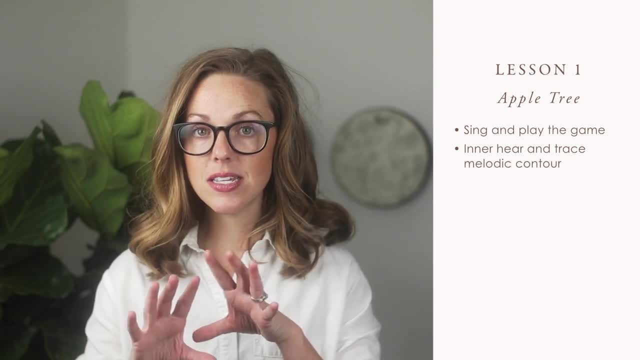 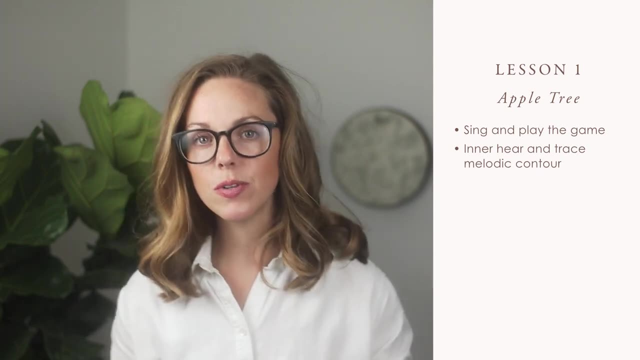 because we're probably teaching the song and the game, since this is the first musical lesson with this concept focus, And then, after we've played the game for several rounds, we'll do a challenge. Students are going to stand in place and hear the song while they trace the melodic. 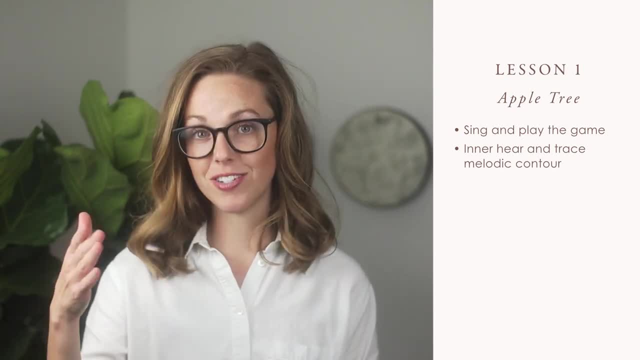 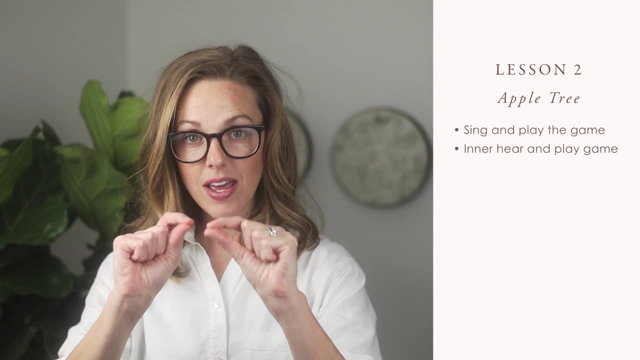 contour of the first eight beats. That's it. That's the whole first day, seven minutes. In the next class we might move Appletree down to the change of pace section and then spend about three minutes on it tops. So for this we'll sing the song and play the game. 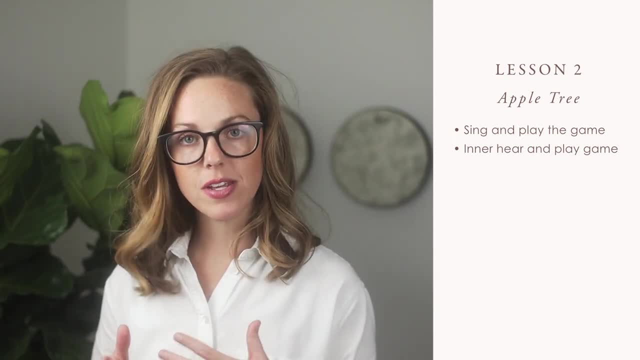 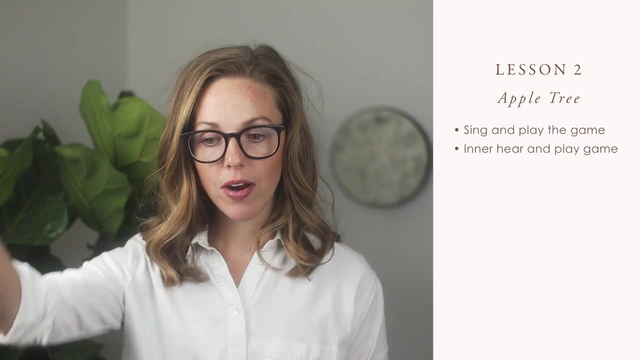 like we did in the first class, And then, after a few rounds, we can challenge students and ask them to inner hear the song while we play the game. If you're not familiar, inner hearing is where it's like you turn the radio on in your head but you're not making any sound. So for this, 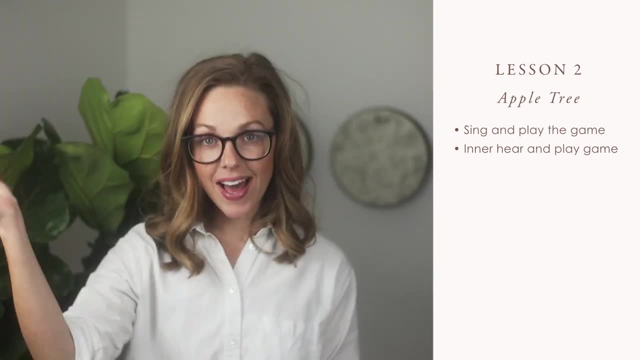 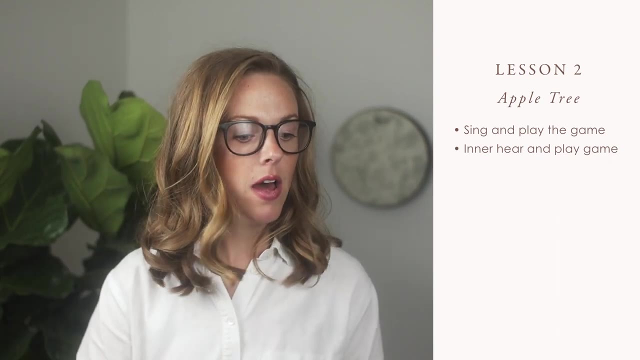 students would have to be all singing the song at the same time as they play the game together, And then in that lesson the main concentration portion of the lesson would be another so lost. so me song like we are dancing in the forest. In the third lesson we can move. 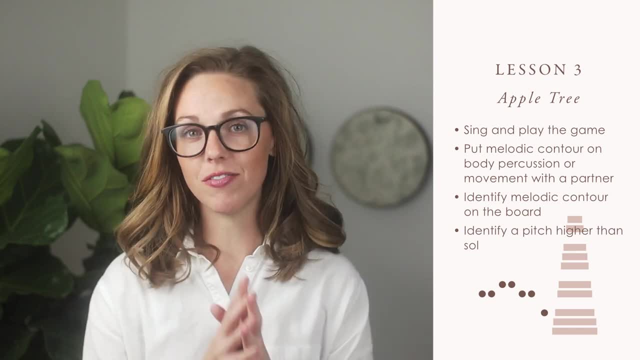 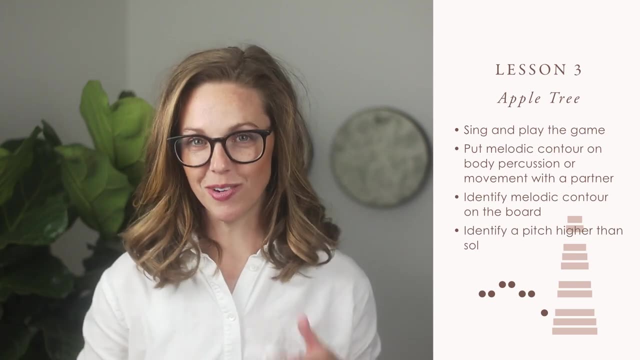 Appletree back to this main concentration section of the lesson And we'll start by singing and playing the game like we've been doing. but we're probably only going to do it once because there's a lot of other stuff to get to in this particular lesson segment. So we sing. 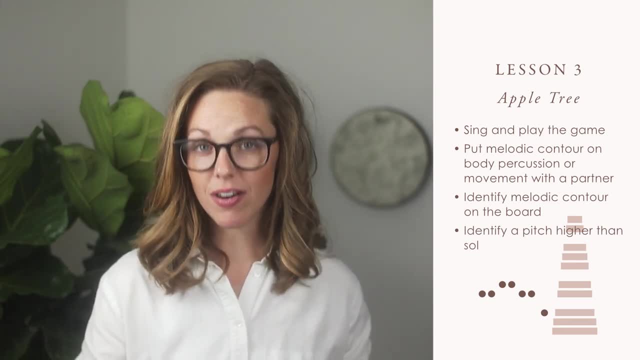 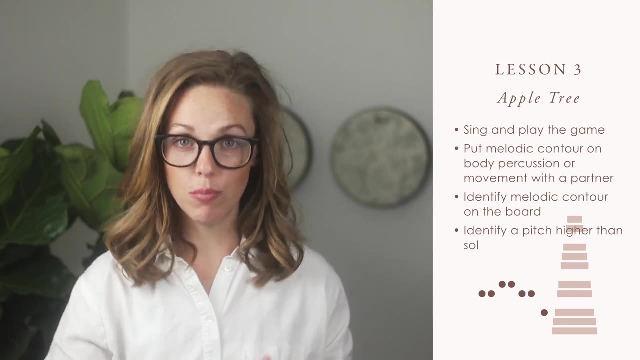 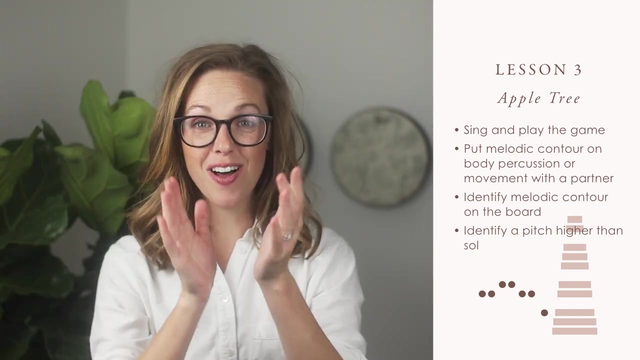 and play the game. And then let's say that we have students turn to a partner and together find a way to arrange this loss. So lost. so me section on body percussion or with movement. So that could be: will your apples fall on me or will your apples fall on me? Lots and lots of options. 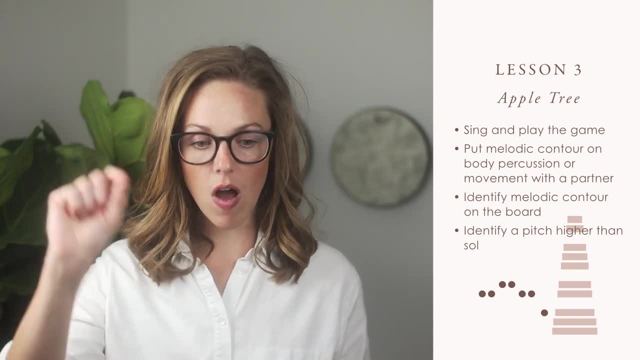 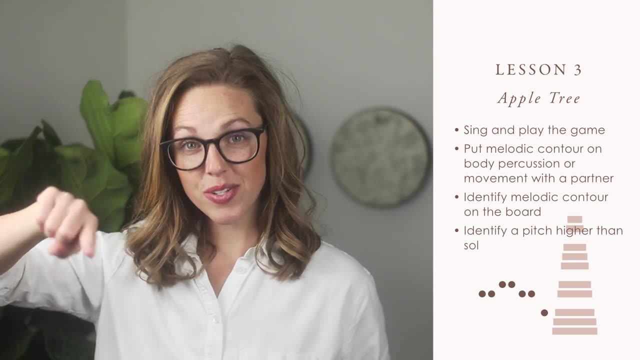 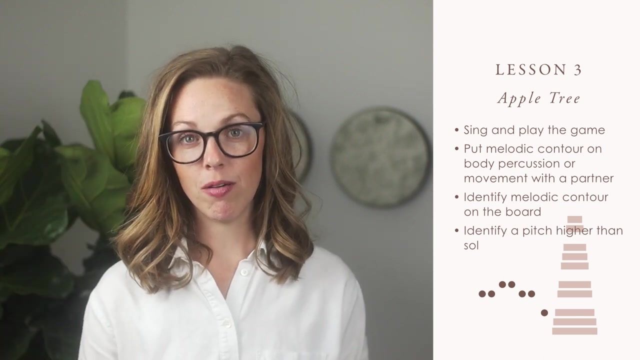 here, And then from there, we might point out the different contour of the melody on the board and trace it while we sing. So we are singing so higher pitch. So me, from there, we can hourly identify that this higher pitch is a step above. So, and by the way, if we were, 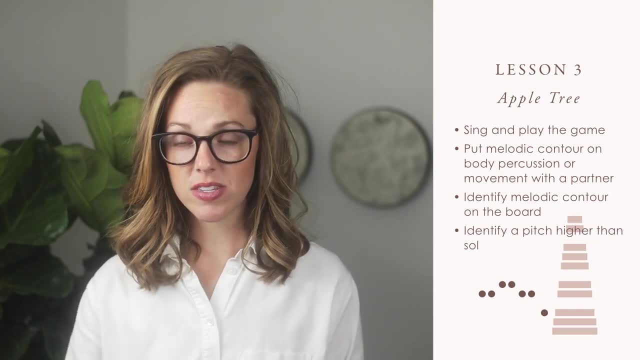 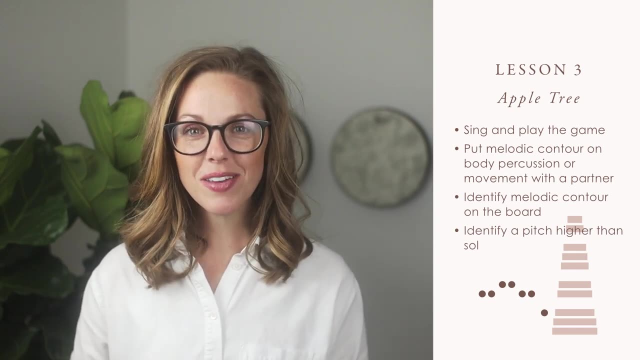 to use a barred instrument for this step. that would make a really nice visual. That's a conversation for another time, but that can be a nice scaffold for this step and skip work. here We can visually identify a step higher than so by the fourth class. we might want to break away. 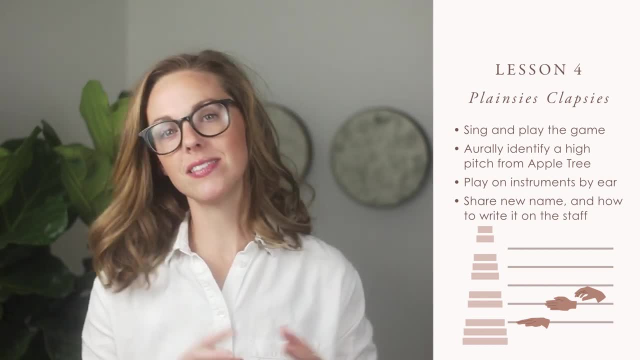 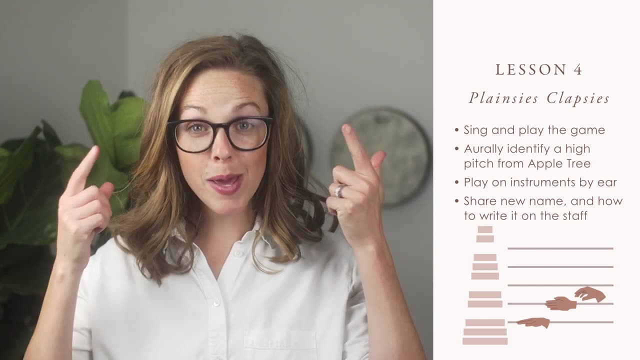 from apple tree. So the main concentration part of the lesson. we can sing the song and play the game too, Let's say planes these classes, And after a few rounds we'll probably discover that this new high pitch from apple tree is in planes these classes too. 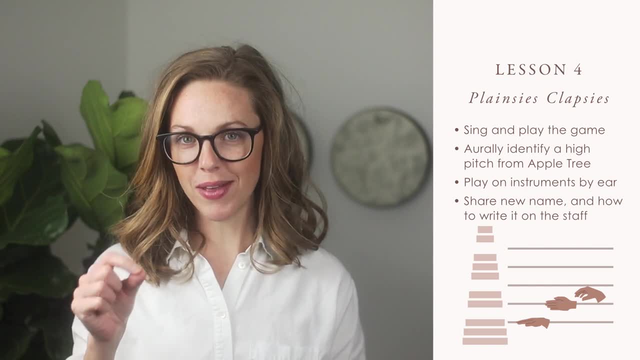 And then from there, instead of us showing students the melody contour on the board, students can show it to us. They can map it out themselves, line by line, And they might even discover that they're not going to be able to do it. They're not going to be able to do it, So. 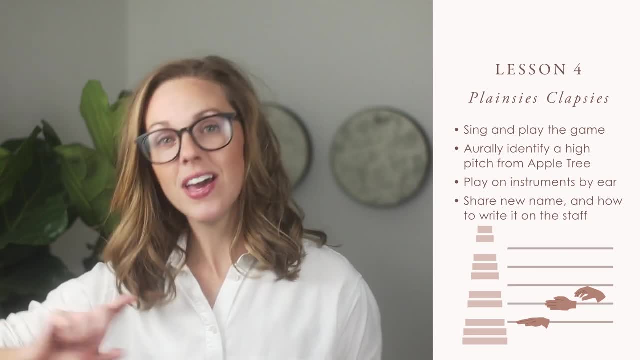 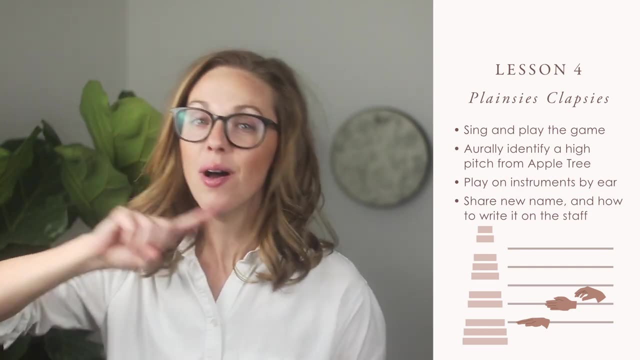 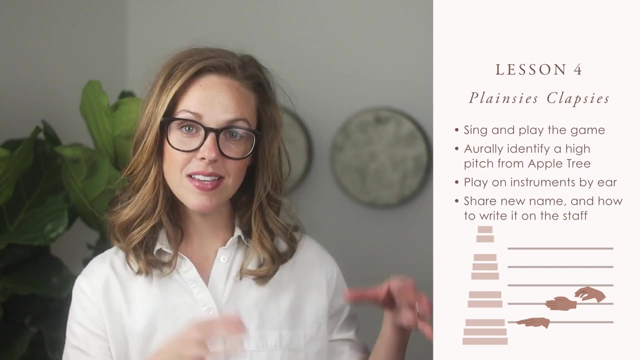 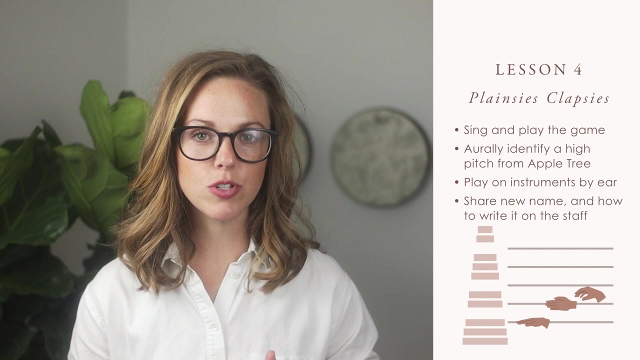 that this same is the same core melody. that happens the entire song, throughout the entire thing, And then, with a partner, students can figure out how to play this song on barred instruments by ear. If it's in line with your pedagogical goals, this might be the time that you change the. 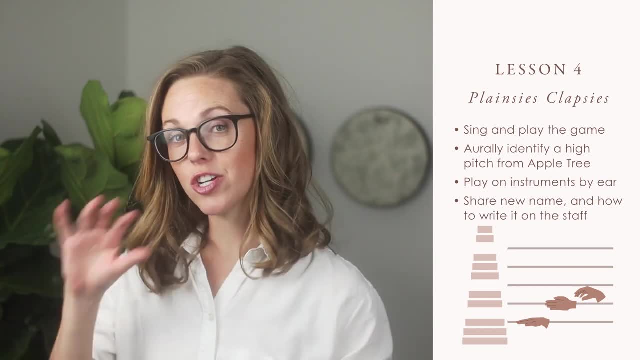 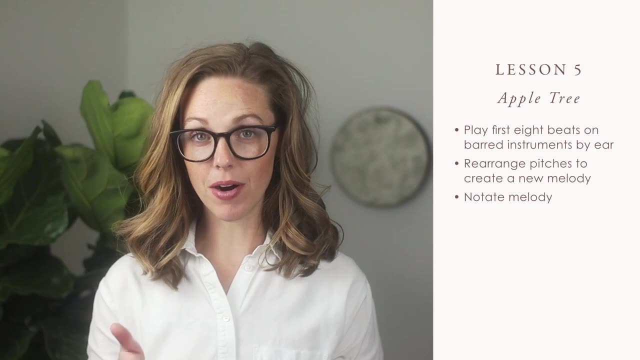 vocabulary from high, this new high pitch to law, and show how you write it down in class. Let's say that we bring apple tree back in the next class and figure out how to play it by ear on barred instruments And then, with a partner, students can rearrange those pitches to create. 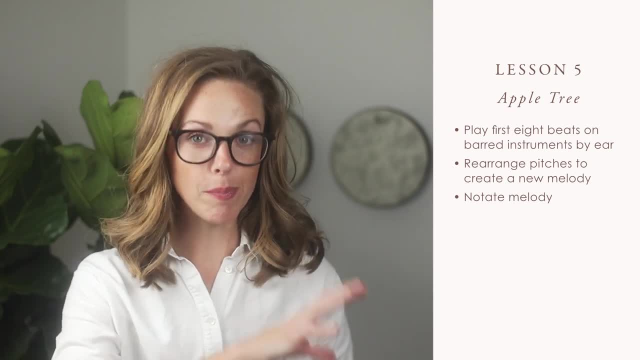 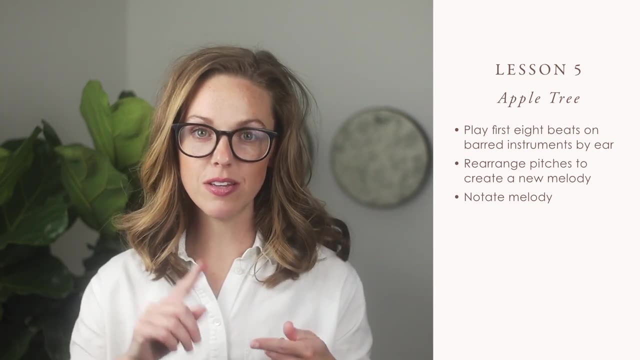 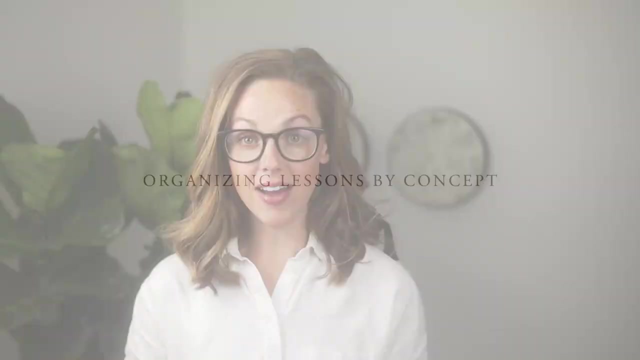 their own version of the song and new melody to apple tree, And then students can use bingo chips or other manipulatives to write down the contour of their new melody, using So me and this higher pitch law. that might sound like a lot, And it is. in these examples, students 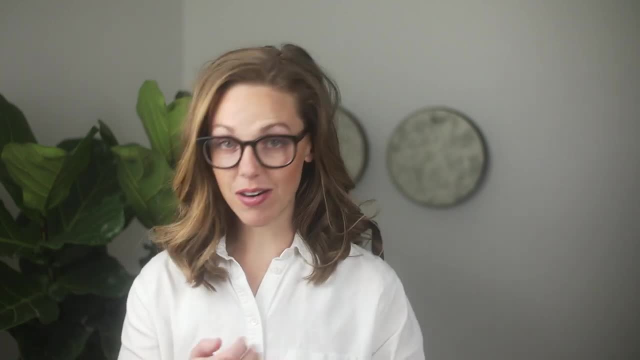 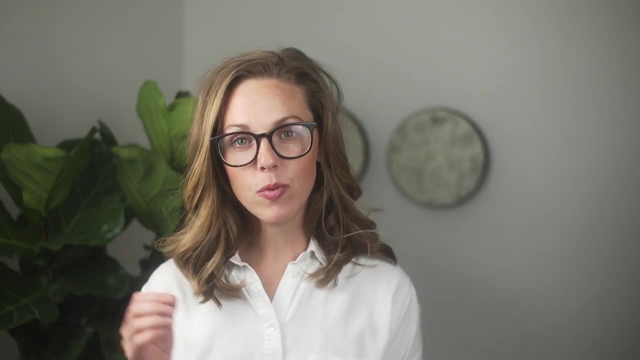 are singing, they're playing barred instruments, they're moving, they're reading, they're writing, they are arranging, they are early identifying their inner hearing and they're playing a game. We also have a lot of collaboration with other classmates and we have creative choices by 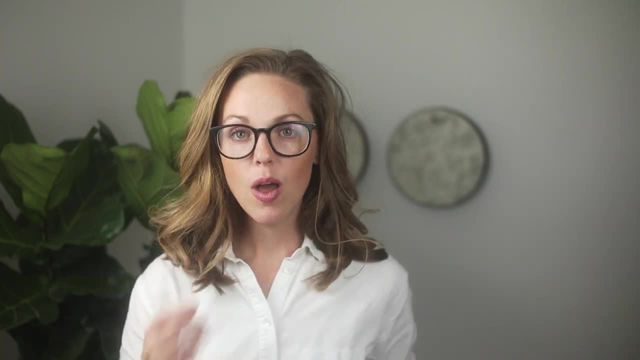 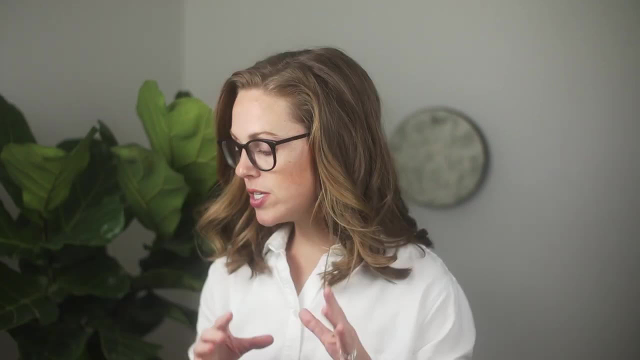 arranging things for body percussion and rewriting the melody. When we look at these lessons there are even more activities here than the activities based lesson structure. But you see we've zoomed out and we are looking at musical skill development over time, not just a single. 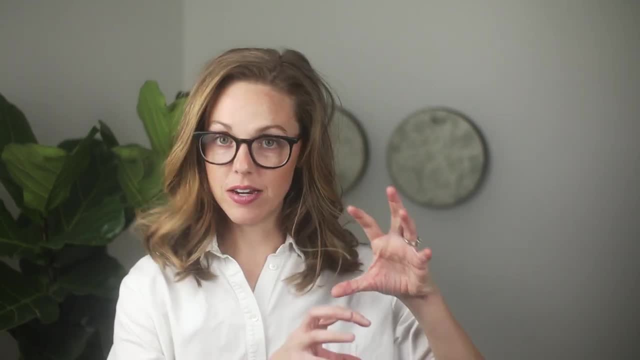 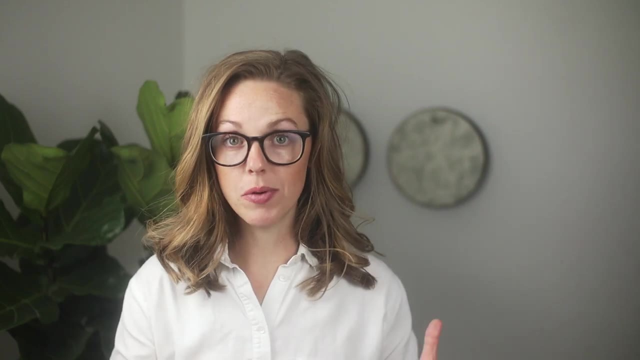 class. So we're looking at musical skill development over time, not just a single class. You'll also see that these skills are not isolated on their own in a specific part of the lesson right. So like there was not a specific lesson segment for arranging, We were just naturally 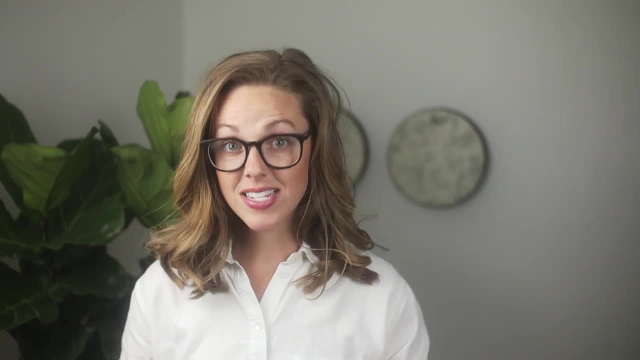 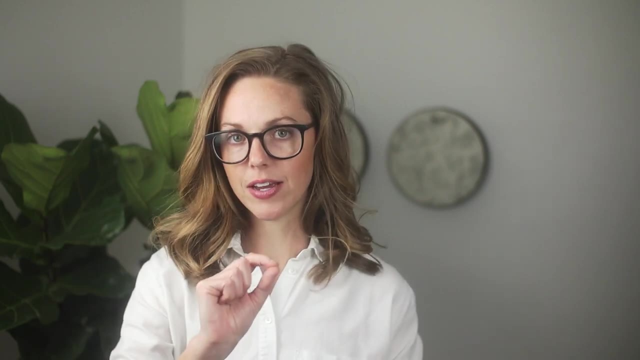 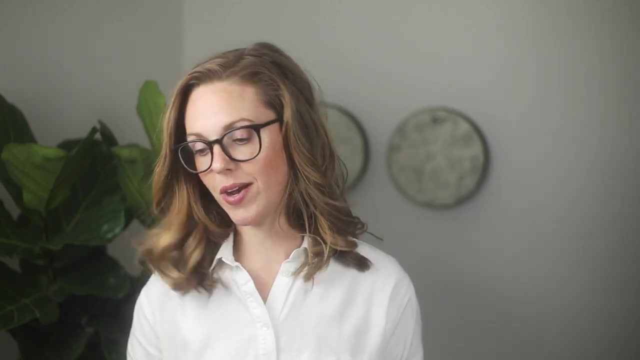 embedding arranging in the learning process, In this case the pitch concept in that specific tonal pattern. so law, so me, because there's a connection between these lessons. over time, students can figure out a song by ear on barred instruments and they can arrange things and they. 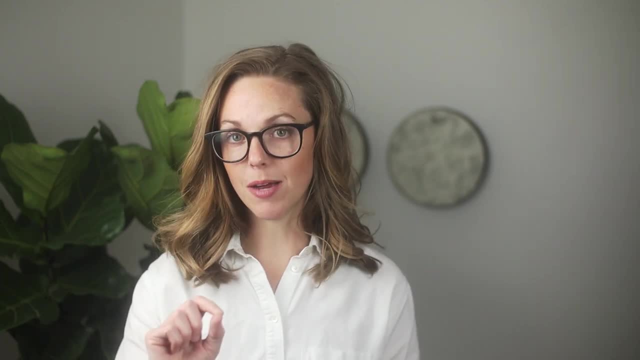 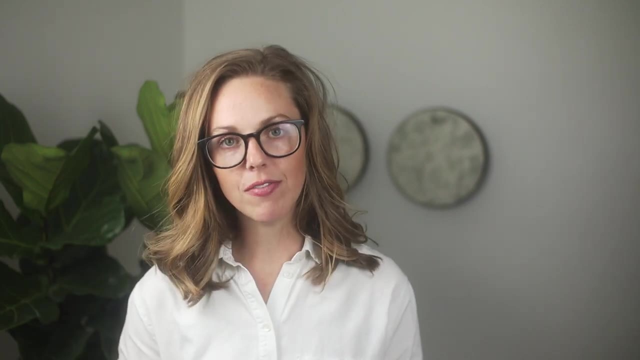 can write them down. So that's a great way to get a sense of the structure of the lesson. They can write down their arrangement because they've been thinking musically about this one specific pitch pattern for lots of different lessons, One way to think about this that I 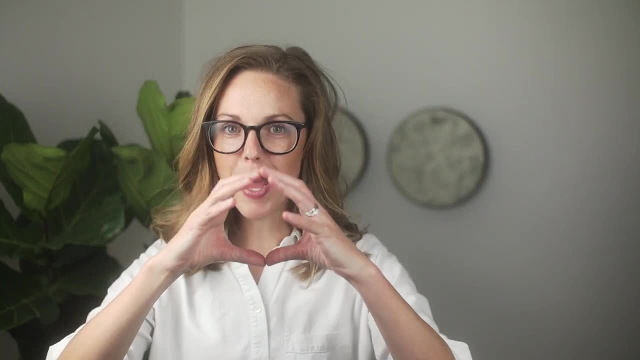 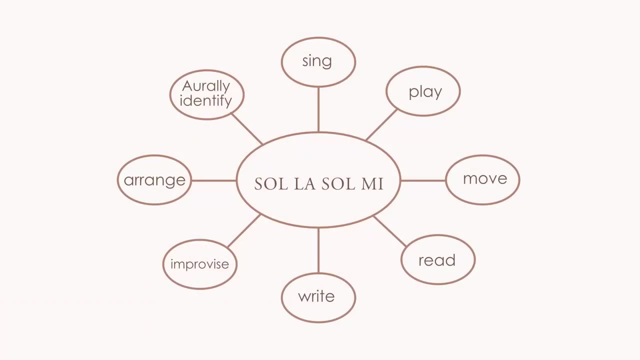 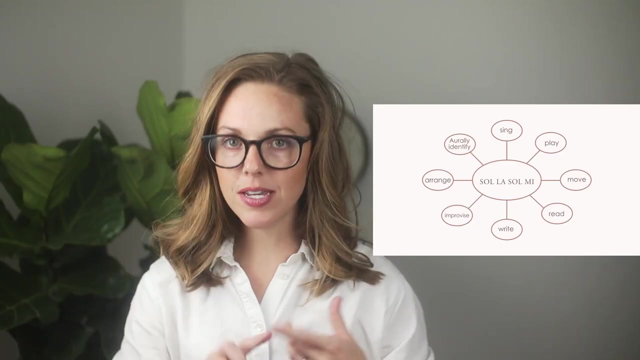 find really helpful is, you know, those bubble mind maps. If we were to take a map like that and put the musical concept in the center, then all of the ways we can show that concept would go around that one specific pitch understanding. So we are, you know, singing and playing and moving, and 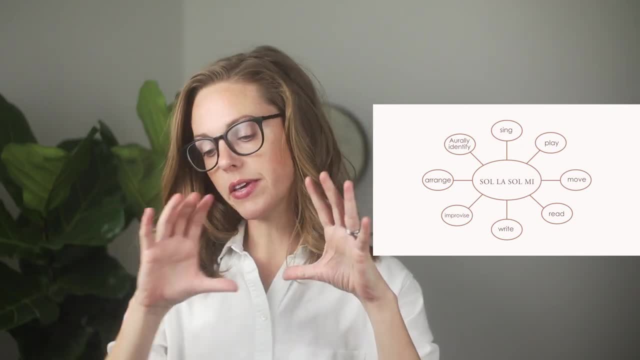 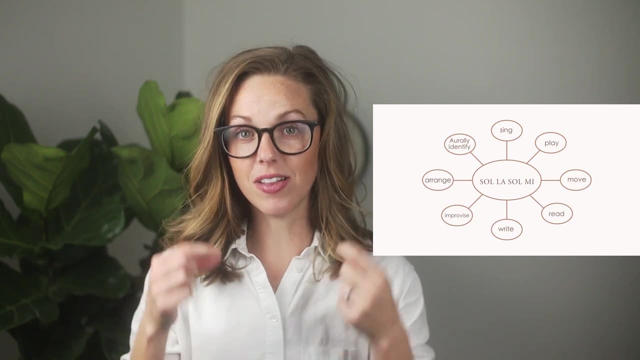 reading and aurally identifying and all of these things. These are all of the experiences that bring diversity to the lesson over time. but notice, they're all pointing back to the same purpose of the lesson segment, In this case, law and so law. so me, The benefit of this is 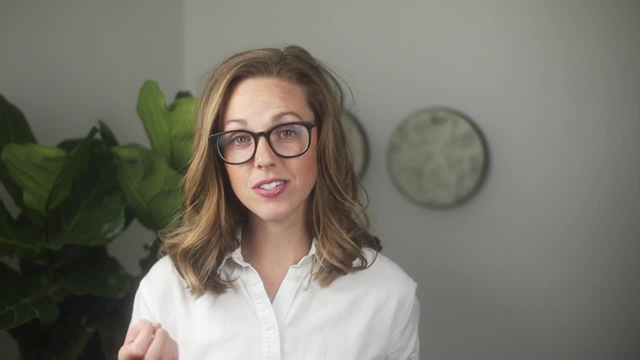 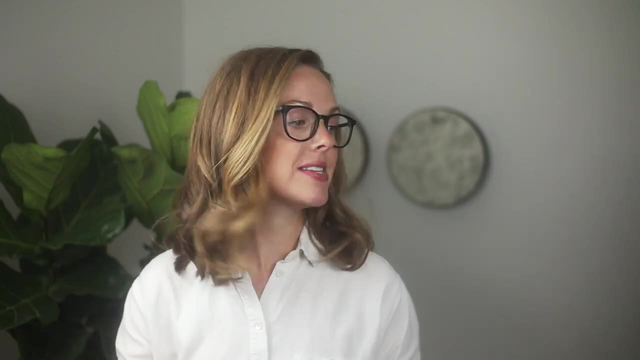 that when it's time to expand our tone, set to include other pitches, students have the aural skills to articulate what they notice about the new pitch. So is it higher or lower than what they already know? Or is it higher or lower than what they already know? Or is it higher or lower? 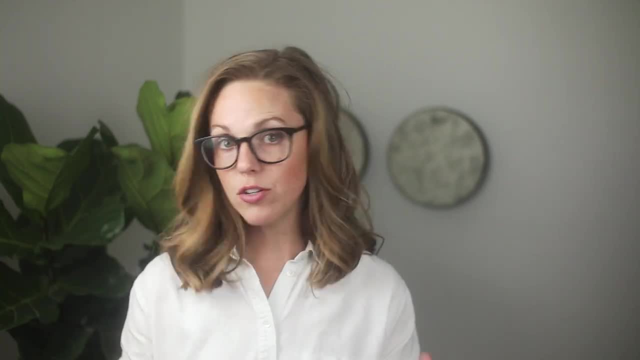 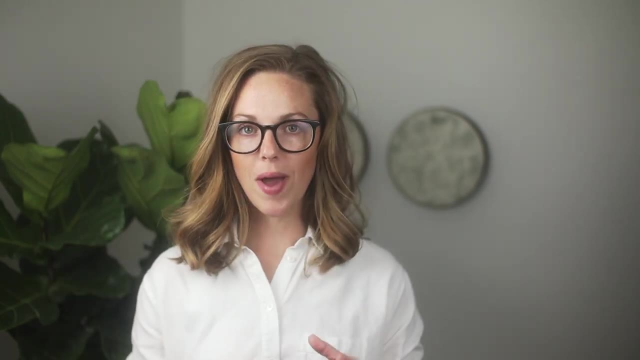 than what they already know? Or is it higher or lower than what they already know? How much higher, How much lower? And then does the new pitch happen in other songs we sing in class or songs that we sing outside of class, When we know how far away it is from other pitches in our conscious. 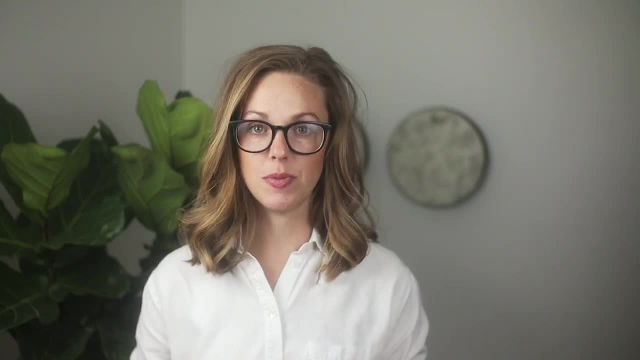 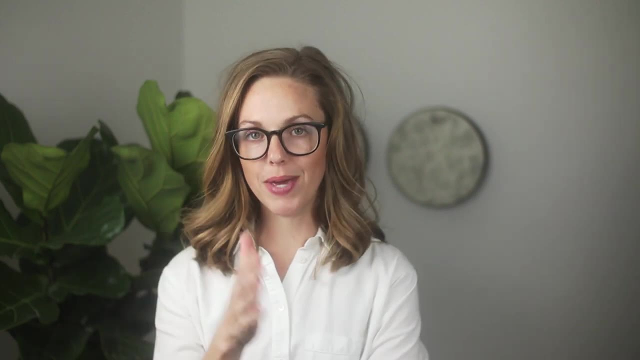 vocabulary. we can figure out songs by ear, on barred instruments or on recorder or on piano or whatever instrument students are using. And that's the beauty of this concept-based approach. In concept-based teaching, we are allowing for the transfer of knowledge between lots of different 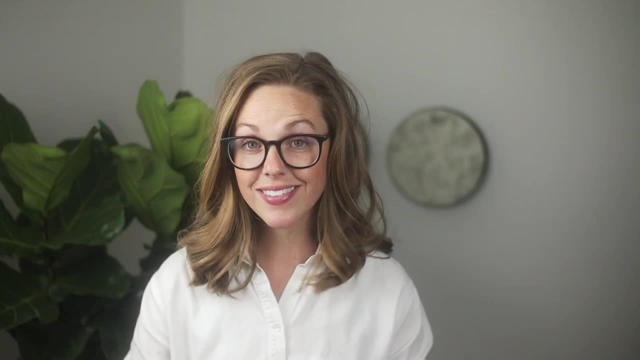 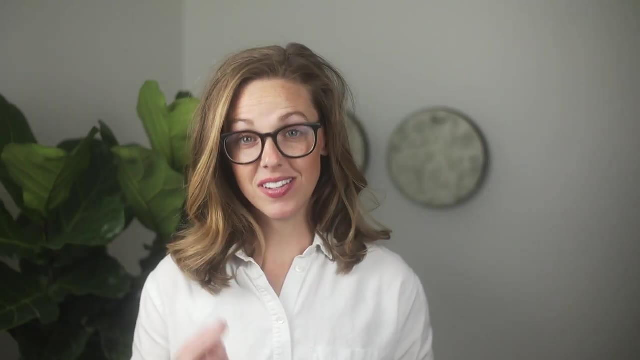 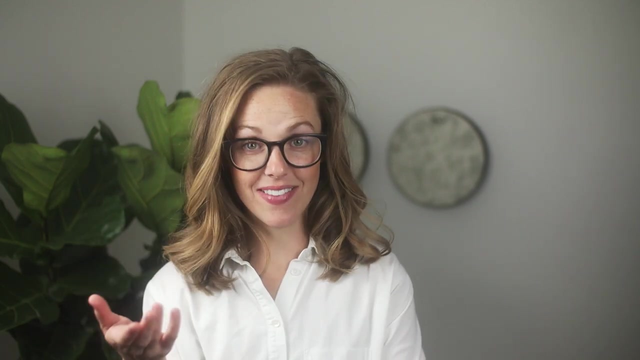 classes, And that can happen in school settings and outside school in the real world. So you can probably see that this way of planning is really closely tied to long-range curriculum plans, And this doesn't mean that we can't search Pinterest for a fun third-grade activity.